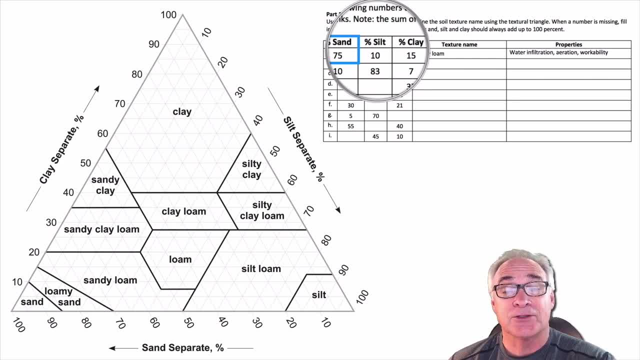 calculated. So 75 plus 10% or, excuse me, 10,, which is a percentage of silt, is 85%. between those two, soil separates. When we take a look at percent clay, that's 15,. 15 plus 85 is 100.. That's how it. 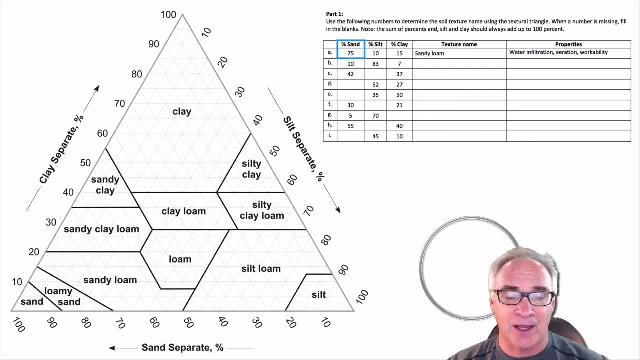 should work. So let's go ahead and draw our first line. It's going to start at the clay- excuse me, at the sand, and that's going to start at 75%. So it's between 70 and 80%. That's where we're going to draw our first line, And when we draw that line, it goes from 75 all. 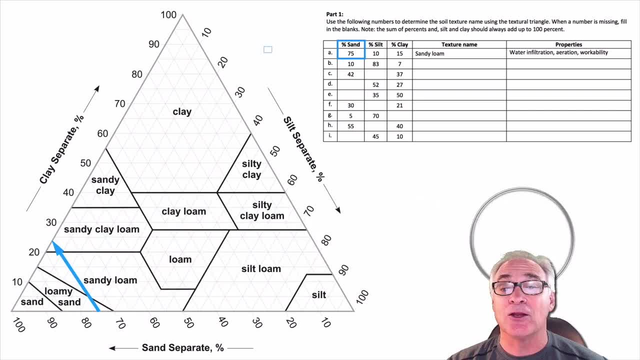 the way to the other side, which is clay. Now what we're going to do is we're going to take a look at the silt side. The silt is at 10%, So we should start our line right here at 10%. So we'd bring. 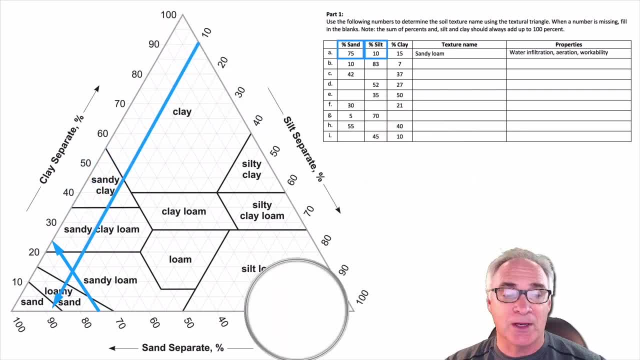 in the line We're going to draw it right to there. So, if you notice, right now we have that intersection of the two of the lines: Sand and silt actually intersect at the line that basically says sandy loam. Now, a loam soil is kind of a loam that's got a little bit of a bit of a. 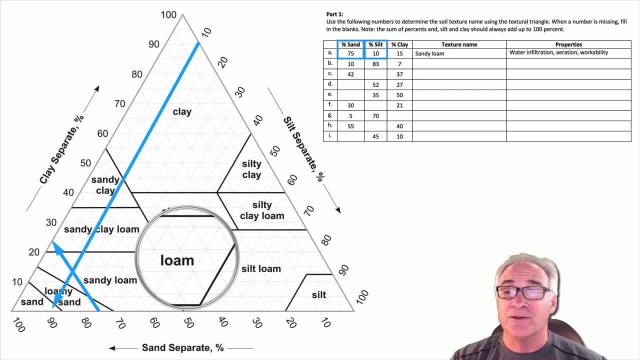 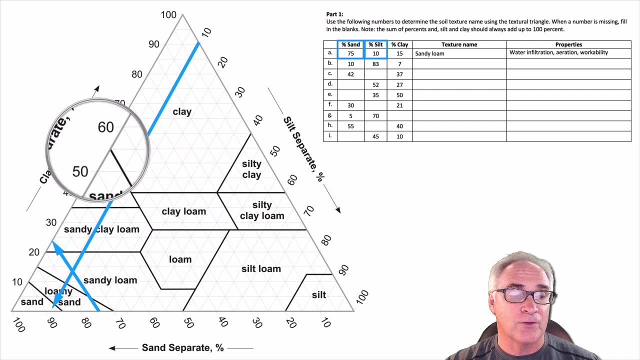 out of the sweet spot. the um, the most ideal kind of of soil has the right amount of sand, silt and clay. this one, obviously. it's gonna have a little bit more sand, but we have to first of all to make sure, uh, we're correct. we have to draw this line at at 15 clay and that's, of course, over here. 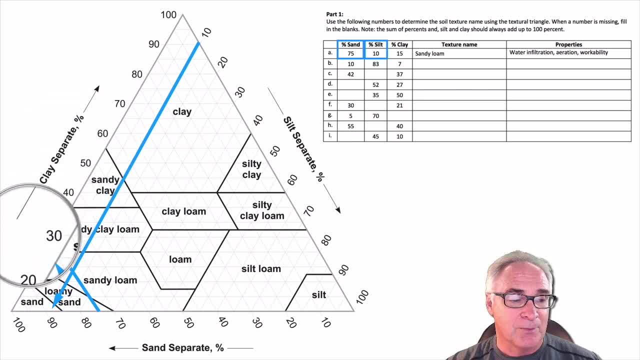 right here on the and the clay separate, and that should be between uh 10 and 20. so let's go ahead and draw that line, and there it is. and now, when with all of those lines intersect, that will be our texture for that sample. so let's take a look. we've left a red dot in its place and it indeed 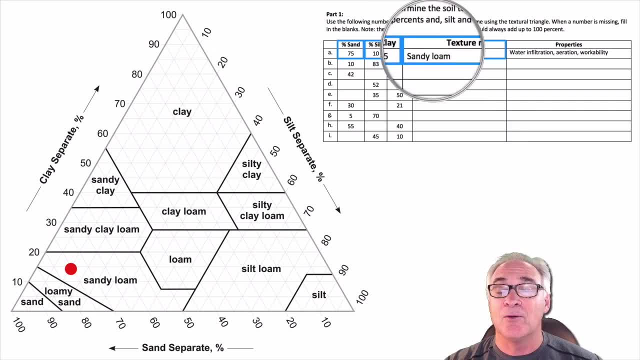 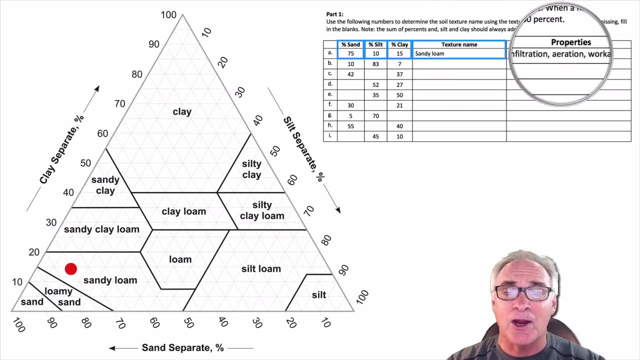 is a sandy loam. so we have a sandy loam and it behaves a certain way, and we're going to be talking a little bit about that at the end of the video today. so let's try one more. uh, this is a sample, number b or letter b, and we have 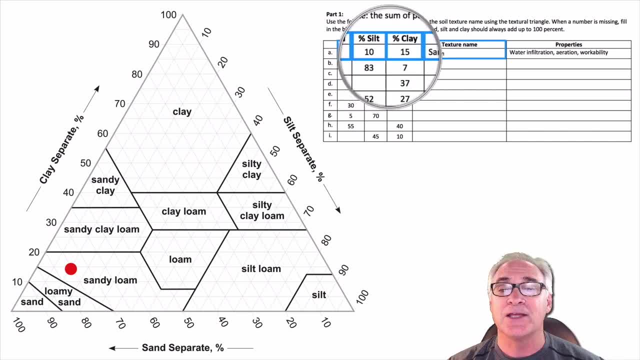 10 sand, 83 silt, and then on the clay side we have seven percent. we add those, all those up and of course it's a hundred percent. ten plus eighty three is ninety. uh, three plus seven is a hundred percent. so let's go ahead and draw the first one, which is sand, at ten percent, and the 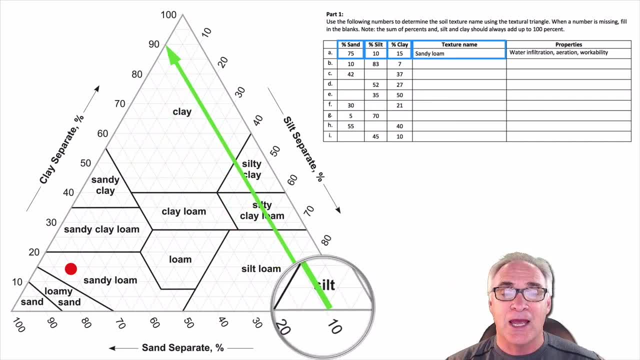 sand is right down here. so we're going to draw that one first and it draws the line straight up to around 90 over on the clay section. then we're going to get on the silt side which is over here, and it's going to be 83. 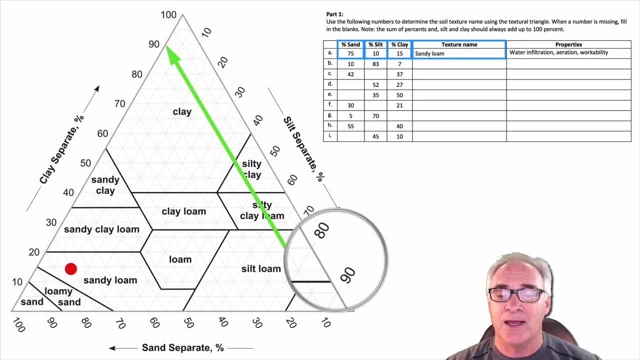 percent, so it should be just past the 80, uh and uh, at least on the 80 percent side, rather than the 90. so we're going to go ahead and do that and notice how those arrows go kind of down. if you notice these little lines here, they kind of help you draw the lines and in this case, right here we. 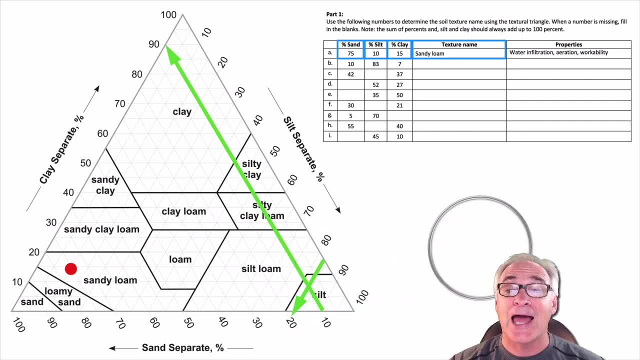 just drew the line straight down to follow that line. and then, lastly, seven percent clay, and that's coming from the clay side all the way over to the silt side, and where those three lines intersect is where we're going to put our dot. uh, for the, the kind of soil that we have. and according to this, 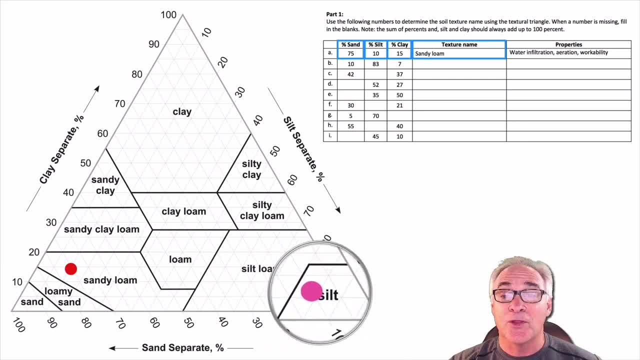 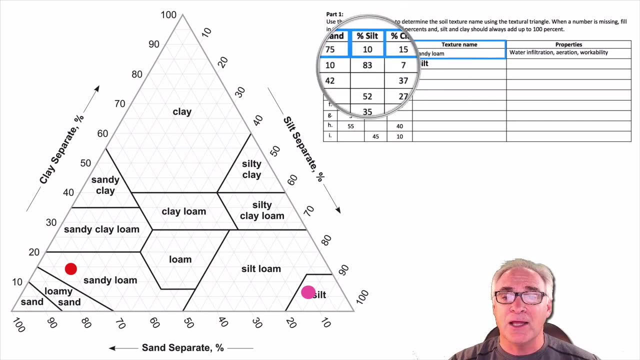 it's silt, it's mostly silt, so that means it's going to be kind of medium in its in its characteristics for water infiltration, aeration and some workability. so, uh, what we have here is we've called the texture a silt. now, on letter c, we have a bit of a problem. we don't have that reading. 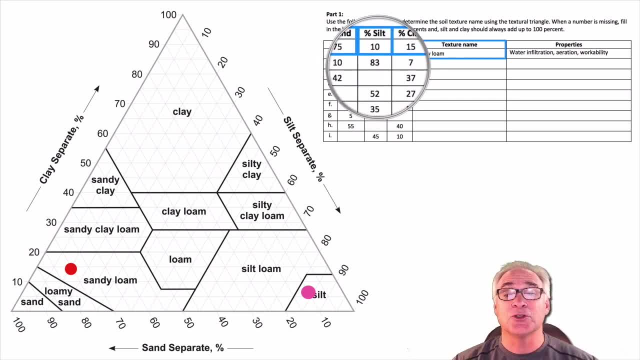 percent of silt, but we have a lot of silt, so we're going to go ahead and do that and we're going to have the other two readings, so let me show you how that works. so we're going to take 42 and then we 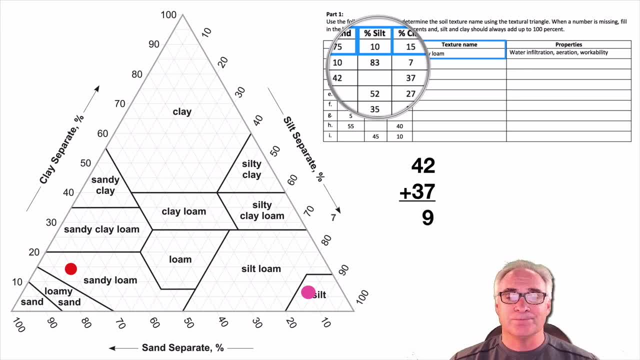 add 37 to it, and when we do that, we get a number 79.. now that is basically the, the sand and the clay added together. now what we need to do is we need to convert that to the silt. so we're going to subtract the 79 from 100, and then what we're going to do is we're going to get this number 21. 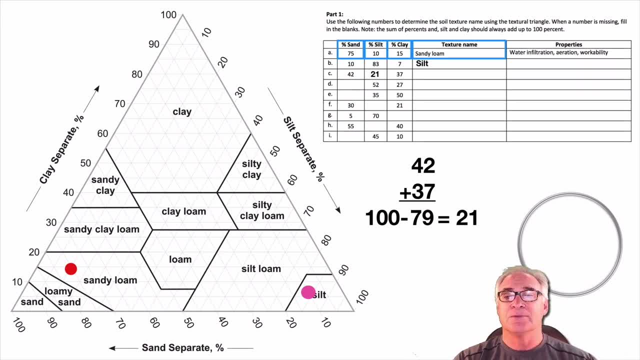 and then we're going to put it right where it is uh done. so, uh, that's what you she will be able to to do, i hope, and um, at least i've given you some helpful hints on how to complete the rest of the chart and then you can draw all the the other. 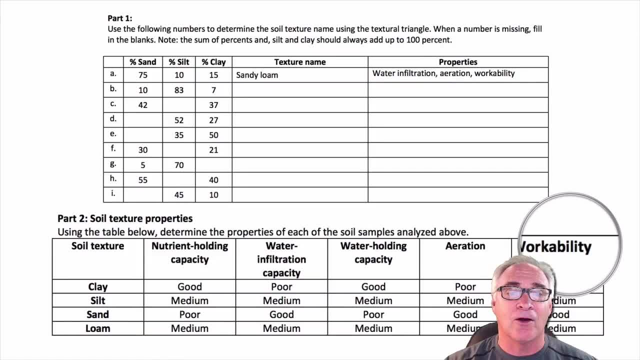 arrows and do it for yourself. so let's take a look at our next thing now. obviously, you're going to be taking care of all of this on your own. now. the next part of this is to figure out what the properties are. there's another um part to this is there's a soil texture, a. 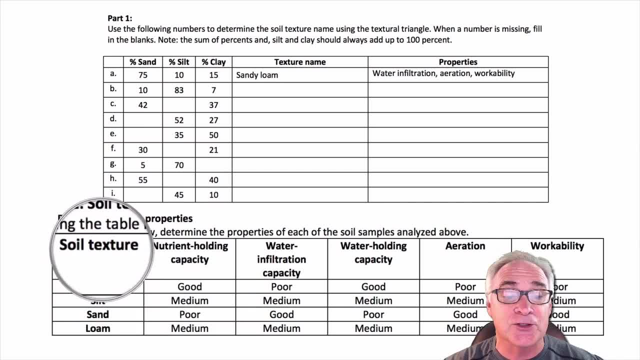 lot of different properties. at the top you have some of the properties that you may have to fill in, from nutrient holding capacity to water infiltration, to water holding capacity, aeration and workability. for this assignment you have three: water infiltration, you have aeration and, of course, you have workability. so let's- uh, let's, do the silt one first, because that was just the. 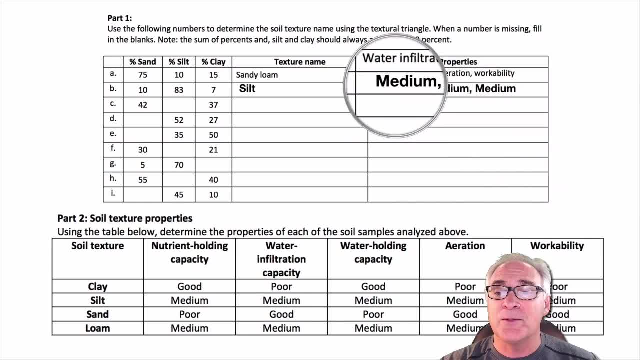 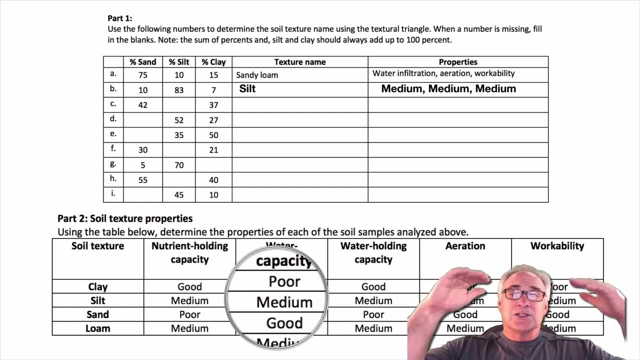 one we just did and if you notice, medium, water infiltration is medium, uh, aeration is medium and workability is, uh, a medium. well, that's because, well, if you look at, uh, right, here we go to silt, it's all medium all the way across, because, remember, silt is kind of the medium-sized soil particle in all the minerals of clay silt. 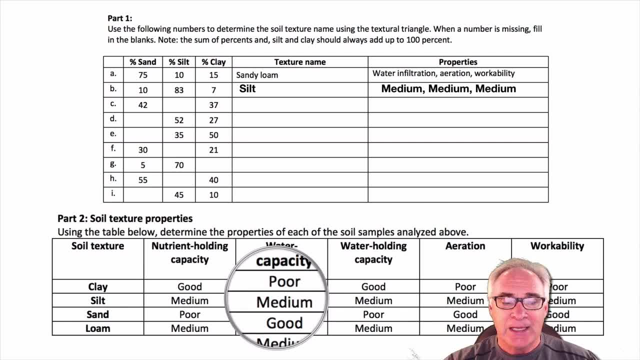 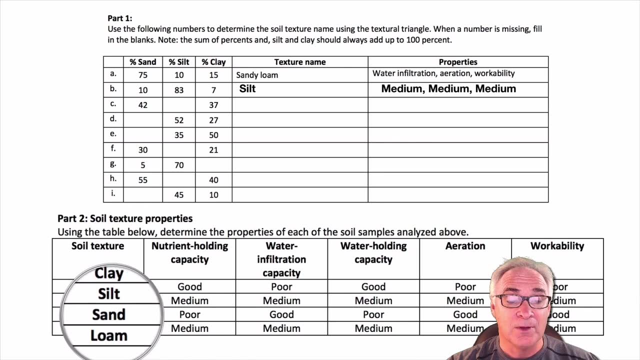 and sand. silt is the one in the middle. and now now, if we were to classify silt, which would be sand and loam, for instance? now loam, as you look down here, is medium and everything kind of like silt. now if you look at sandy loam, it's going to be kind of somewhere in. 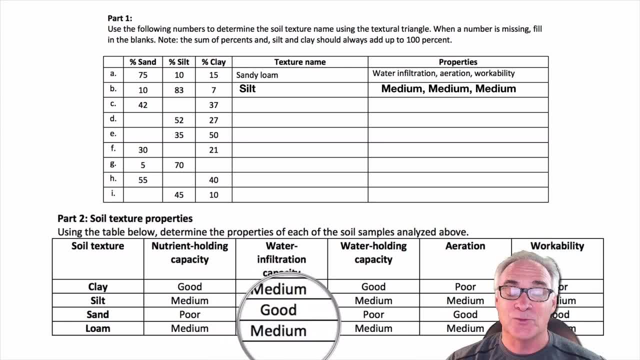 between of all this. so because i've worked in um sandy and long soil before, i can tell you that the water filtration is just that between a good and medium. mostly more in the medium side um of goes through the soil profile relatively quick. As far as the aeration is concerned, it's pretty good. 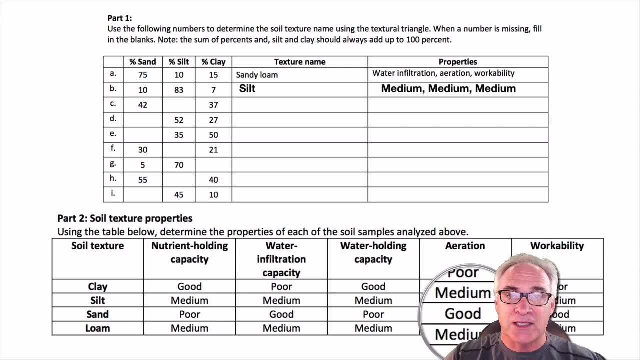 It's kind of more on the good side Because it drains fastly, air can get into the pore space much more easily. Workability: I would also consider that more on the good side than the medium side, because even after a heavy run you can get equipment in and work the soil fairly quickly within.